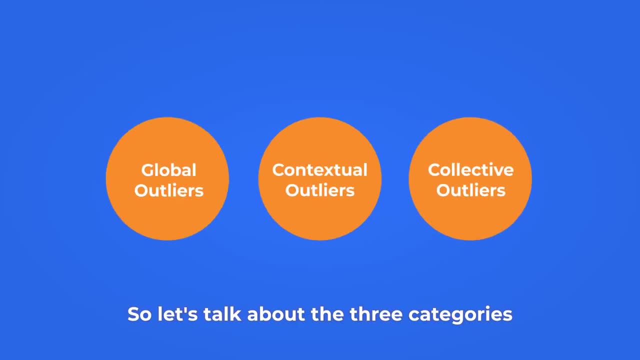 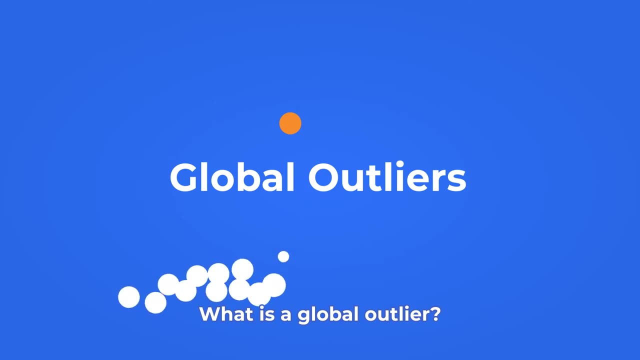 and yields much better results. So let's talk about the three categories that outliers fall into. The first one is called global outliers. What is a global outlier? Well, a data point or points are considered a global outlier if their value is far outside everything else in the data set. 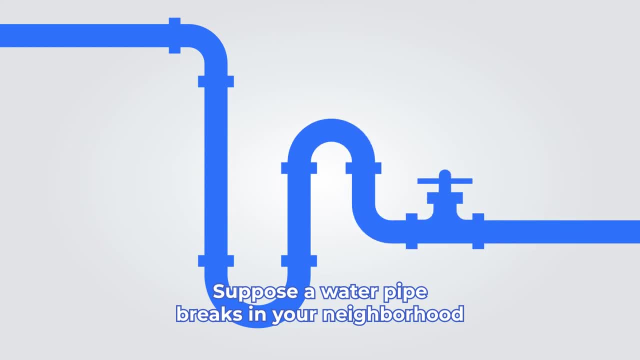 Think of it this way: Suppose a water pipe breaks in your neighborhood, causing your area's water consumption to go through the roof. Well, if you compare it to water consumption in all other days of the year, this would be a global outlier. But let's look at a global outlier in an actual 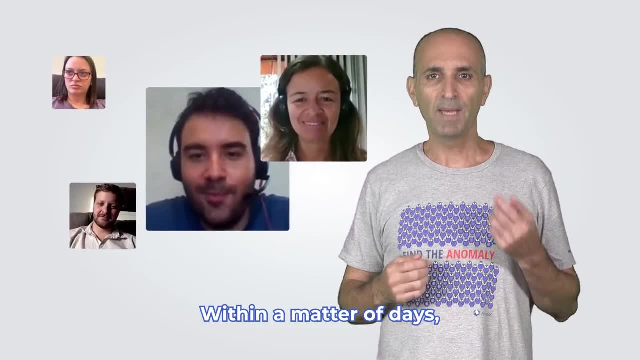 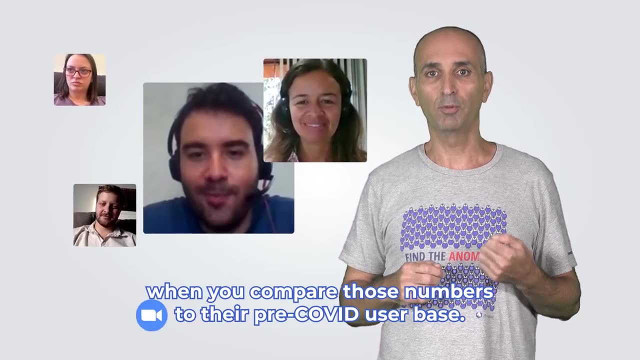 business setting. Think about Zoom. at the start of the pandemic, Within a matter of days, the number of people using Zoom spiked exponentially. That was a global outlier. when you compare those numbers to their pre-COVID user base, This is the ultimate example of a global outlier in a business setting. 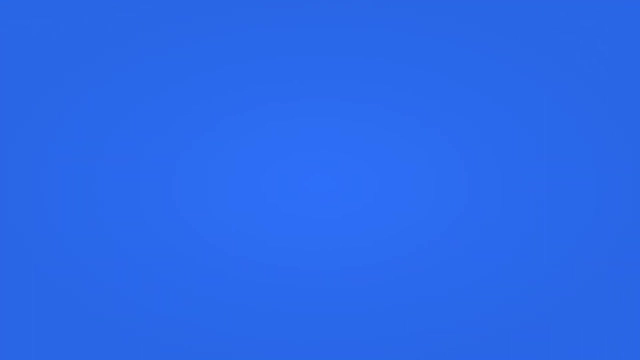 Any business would love that. The second category of outliers is contextual or conditional. A data point is considered a contextual outlier if its value deviates quite a lot from the rest of the data points that are in the same context. Note that the same value may not be considered an. 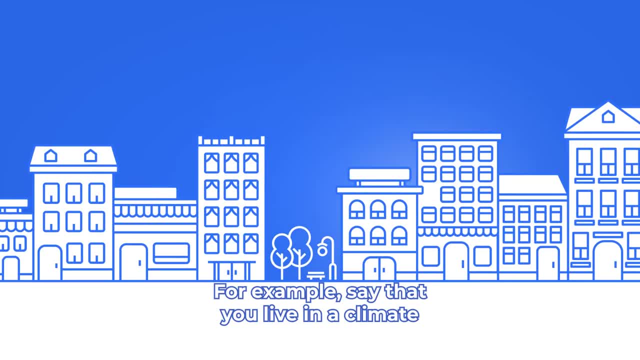 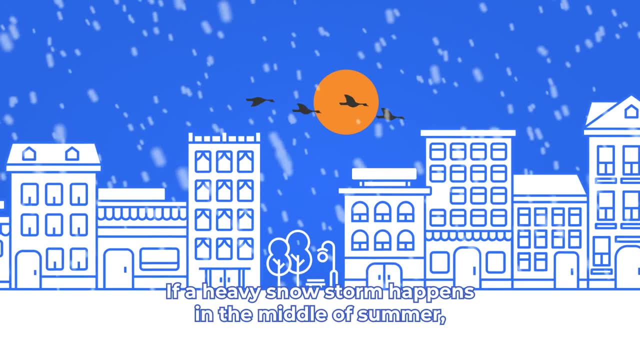 outlier if it occurs in a different context. For example, say that you live in a climate where your city gets snowstorms in the winter months. If a heavy snowstorm happens in the middle of summer, it should be considered a contextual outlier. The event is anomalous compared to the seasonal pattern. 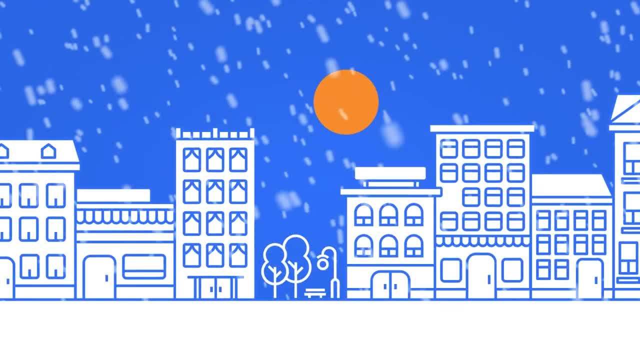 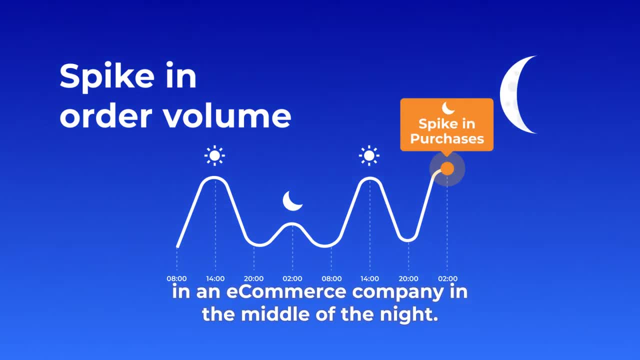 where it typically snows in winter but not in summer. We also see contextual outliers in business. Consider a sudden surge in order volume at an e-commerce company in the middle of the night. It's a contextual outlier because you wouldn't expect this high volume to occur outside daytime. 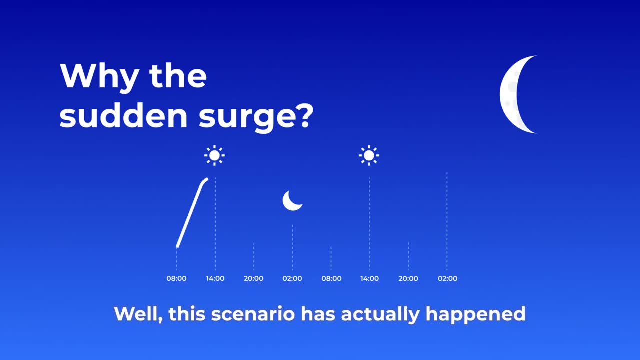 Could this rush of sales be due to a pricing glitch? Well, this scenario has actually happened several times with airlines. It's a very common trend. It's a very common scenario that a company can get out of business that offer tickets- flights- at wildly discounted prices. 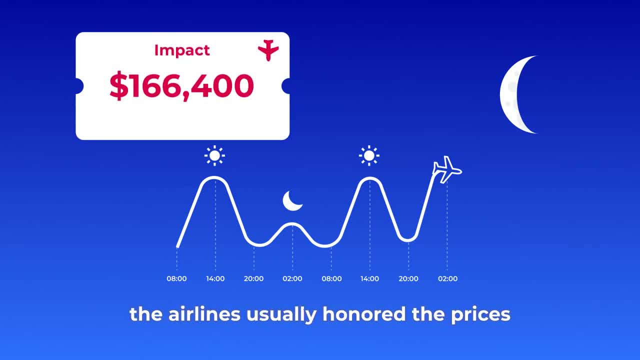 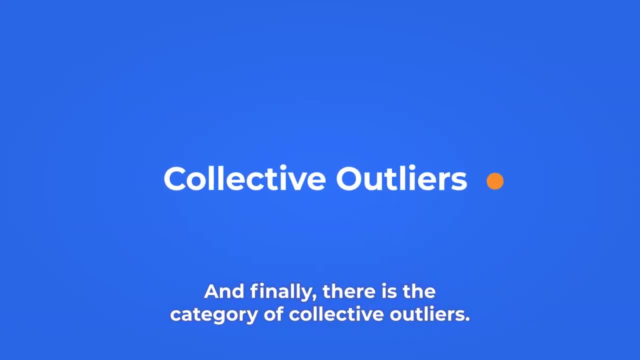 Though the offerings were a mistake, the airlines usually honored the prices and lost significant revenues on those seats. And finally, there is the category of collective outliers. This one's a little tricky to explain. We see collective outliers when a group of data points within a larger dataset.